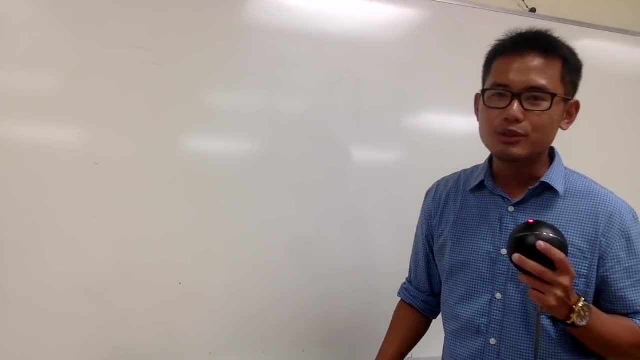 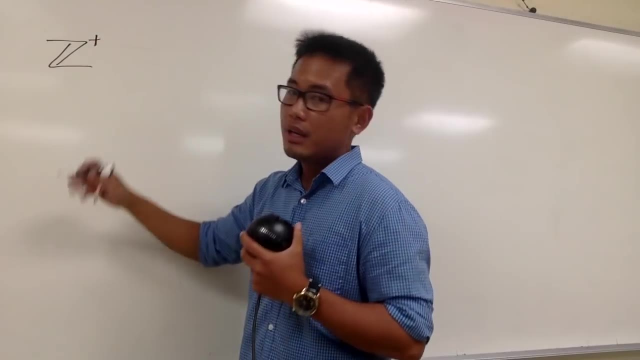 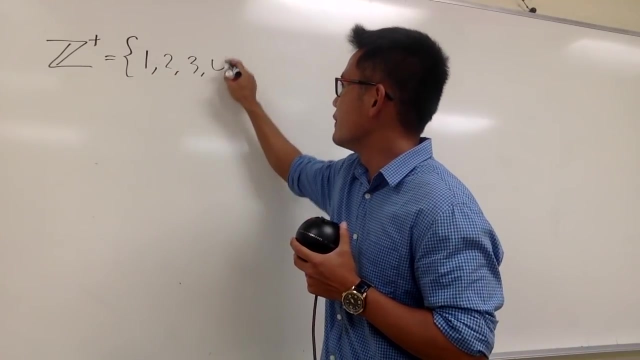 Okay, let's take a look at the set of all the positive integers. In notation I will write this down as z, And because I just want to have the positive integers, so let me put a plus right here. So this right here is just the set of all the positive integers. Namely, we have 1, 2,, 3, 4,, 5,, 6,, 7,, 8,, 9,, 10,, 11, so on, so on, so on, right. 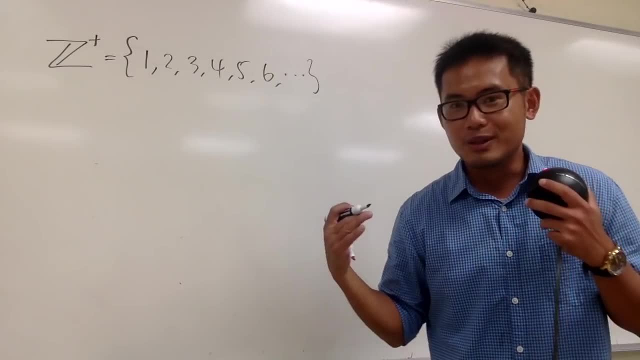 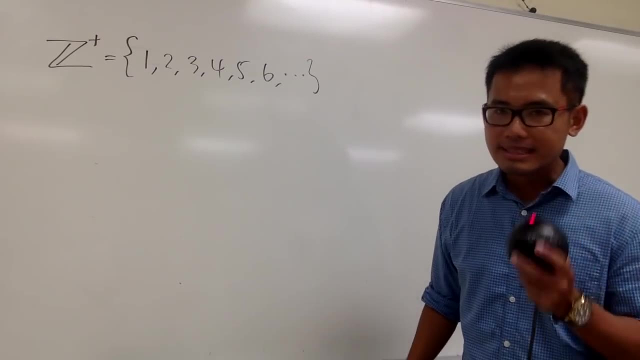 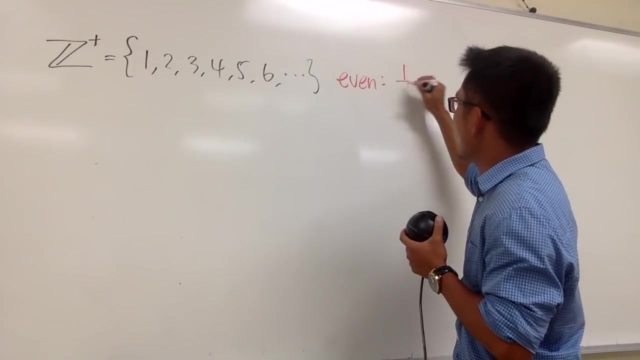 And as we take a look at this, it's also a well-known fact that an integer is either even or odd. So if you look at this, if you want to ask yourself what percent of the positive integers is even, Well, we know this right here is just going to give us 1 half or 50%, right? 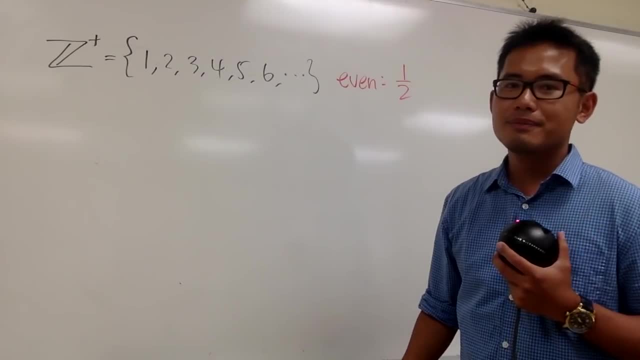 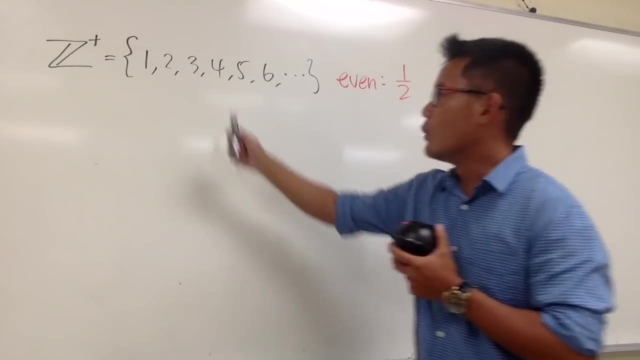 Okay, how about the following? First of all, you guys should agree with me that this is a way to list out all the positive Integers right: 1,, 2,, 3,, 4,, 5,, 6,, 7,, 8,, 9, so on, so on, so on. 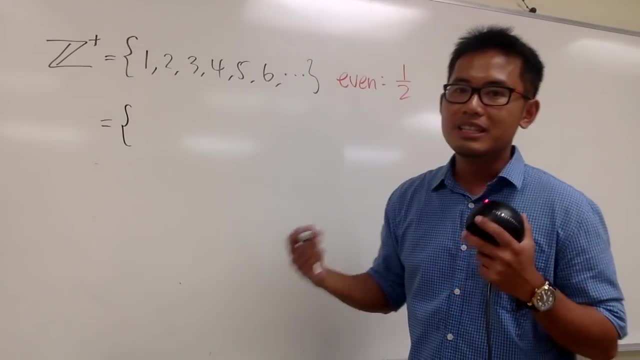 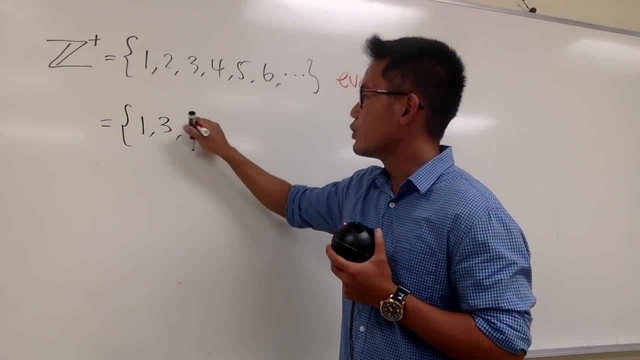 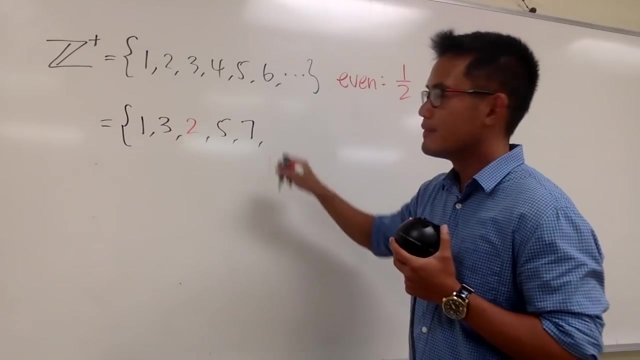 How about if I take a look at the set of the integers this way? Let me write it down as the following: Let me put down 1, and then 3, and then 2.. Okay, so 1,, 3,, 2.. And then I'll put down 5, and then 7, and then 4.. 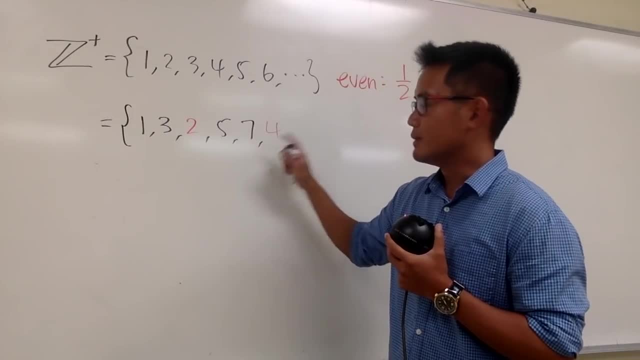 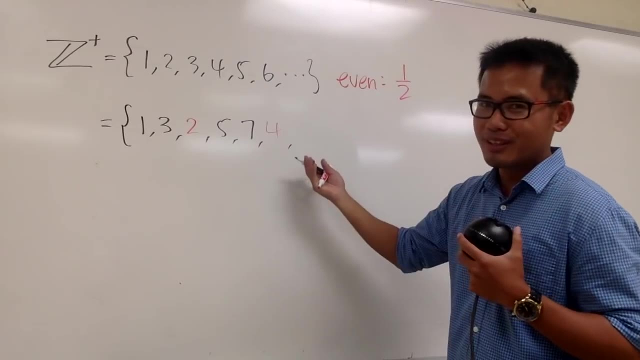 So far, you see I have 1,, 2,, 3,, 4,. 6 is coming out, Don't worry. 5, 7.. If you want to have the 6, you'll see What should I put down. next I will have to put down 9,, 11, and then 6,, right. 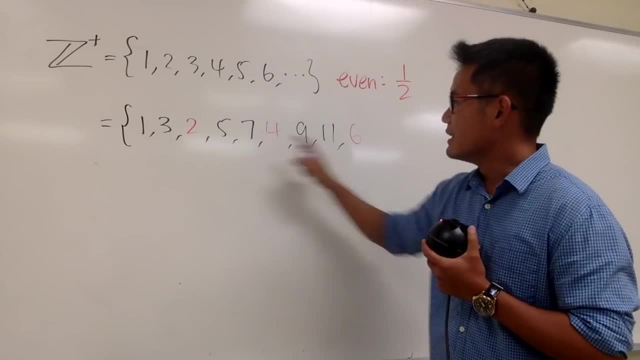 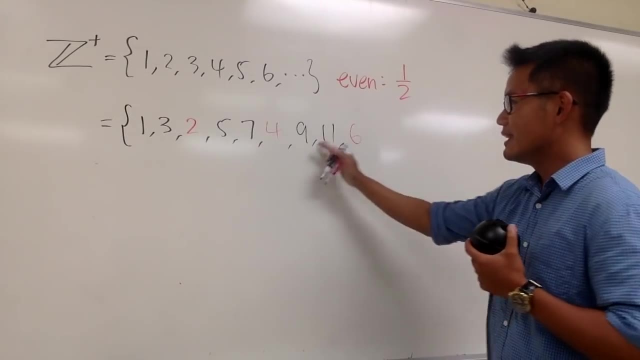 So, based on this, you have 1,, 2,, 3,, 4,, 5,, 6, and 8 is somewhere here, right? I mean 7, and then 8, and then 9, and then 10, and then 11,, and so on, so on, so on. 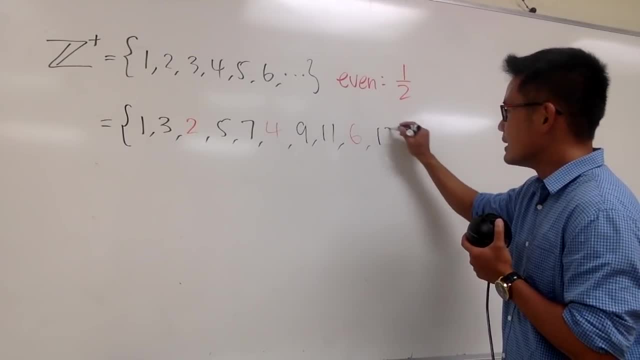 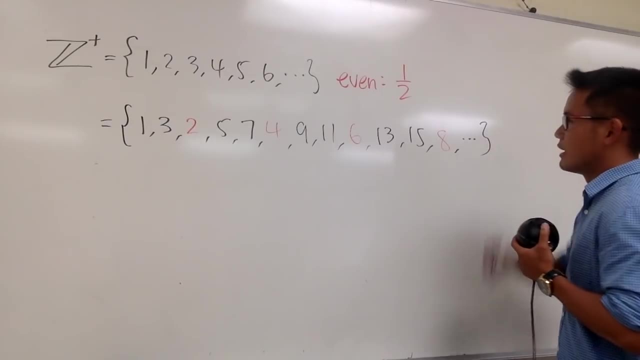 And, if you really would like, let me just do a few more for you guys. The next one will be 13,, and then 15,, and then here is the 8,, and I will just keep the same pattern like this, going on forever. 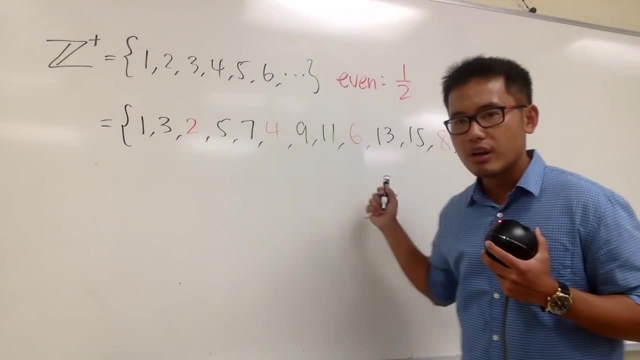 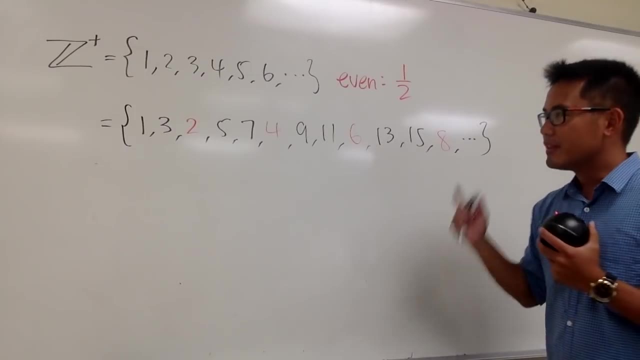 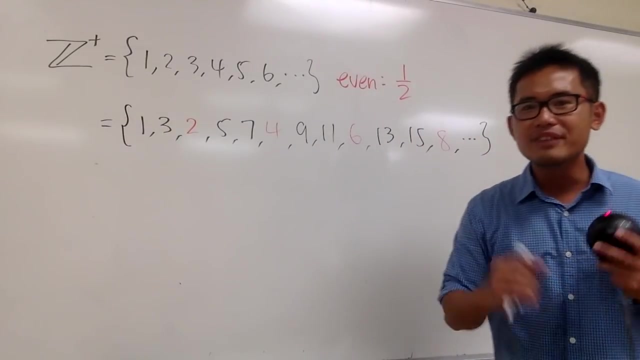 And you guys should also agree with me that this right here is the set of all the positive integers. right, Because I can list them out like this: And now, if you take a look of this list right here, what percent of the positive integer is even now?